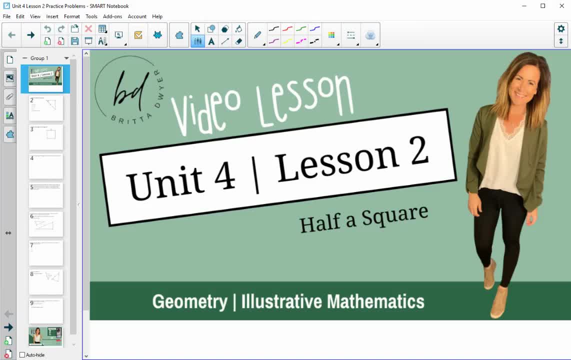 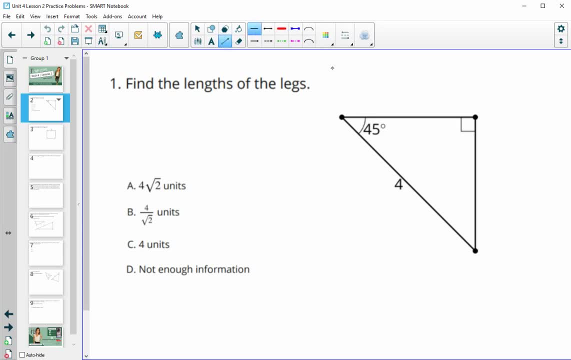 In this video we are going to take a look at the Unit 4, Lesson 2, practice problems. Number one wants us to find the legs of this right triangle shown, And so when we're looking at this right triangle, hopefully you notice that not only obviously it's a right triangle, 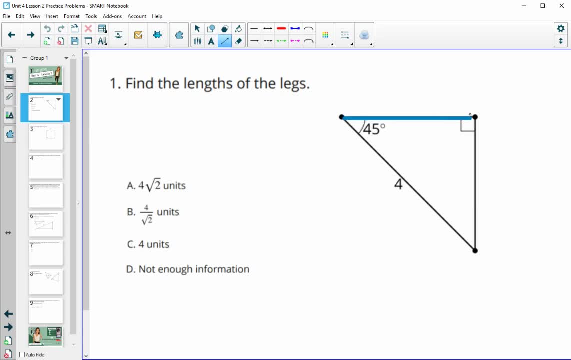 but then also one of the angles is 45 degrees, And so what we learned is: if we have a right triangle and one of the other angles is 45, then that leaves 45 degrees left over for this other angle as well, And then that makes it an isosceles right triangle. 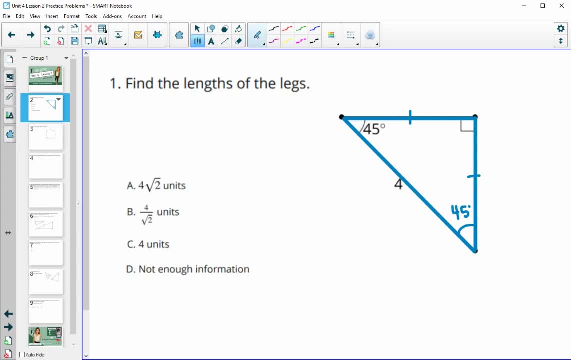 So these legs right here are the same length as well, So this allowed us to know that this is similar to every other 45-40.. So this is the 45-90 right triangle, And so if you kind of take a look at one that I call the parent right triangle, 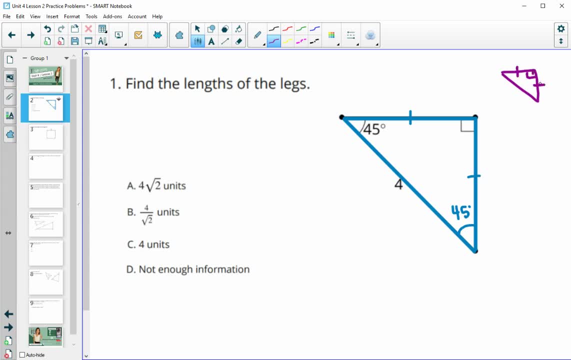 the parent 45-45-90 triangle. this one has legs of 1, 1, and square root 2.. So this is the one that all other triangles, all other 45-45-90 triangles, are similar to. And so if we take a look at this with the scale factor- and you can kind of do it between the sides- 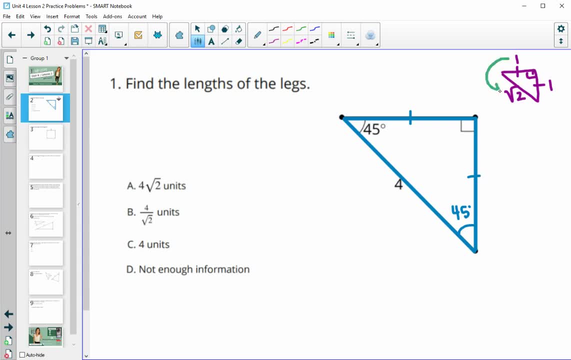 So if you have The side length to get to the hypotenuse, we can see that we just multiplied 1 by the square root of 2.. Now if we had the hypotenuse? so if we knew the hypotenuse. 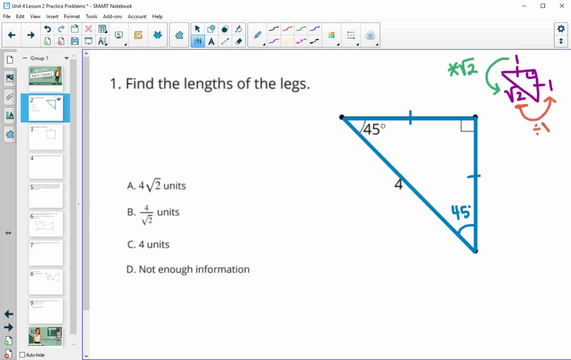 then we take it and we divide by the square root of 2 to get to the leg, And this will work in every 45-45-90 right triangle, And so in this one we have the hypotenuse given to us. 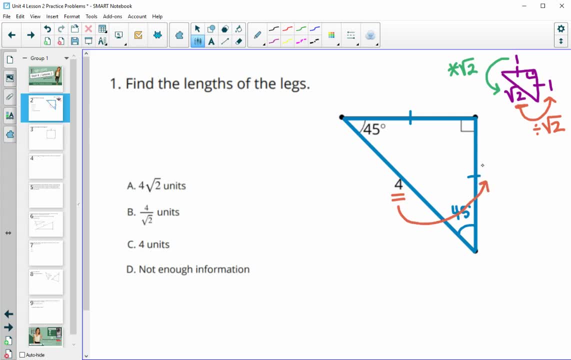 So if we take it and we divide by square, we'll get the length of this leg. So let me just call the leg x here. And so x is going to equal 4 divided by the square root of 2.. And so in our answers here we see that that's actually written as a fraction in part b. 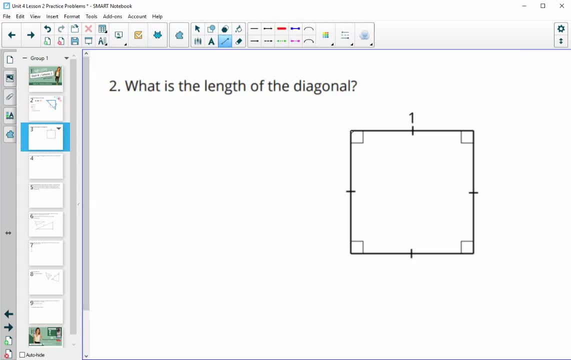 Number 2 wants us to come up with the length of the diagonal of this square. So when we cut a square, we get the length of this square Squares. when we cut a square in half, with its diagonal, it creates two 45-45-90 triangles. 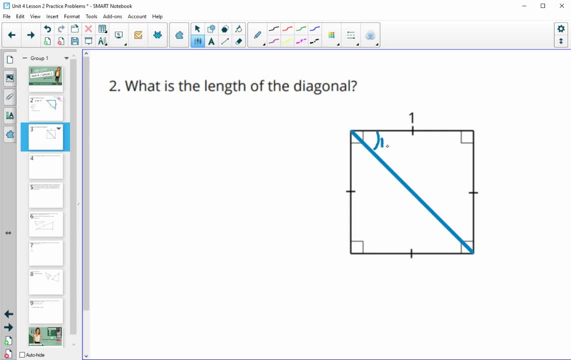 Since we've got the legs the same, that forces these two angles to be the same, which would force them to be 45 degrees. And so now, if we want to go find the length of the diagonal, now we have the length of one of the legs. 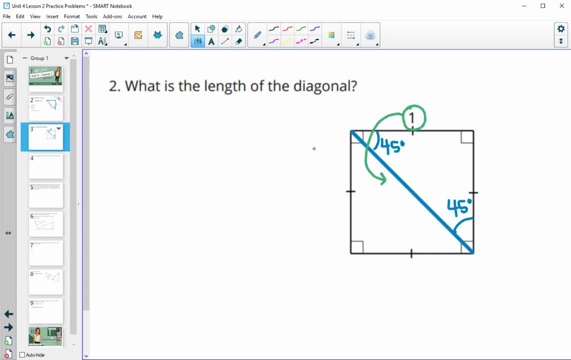 And so when you have the leg you multiply that times the square root of 2 to get that hypotenuse. So if I just call this hypotenuse x, x is going to equal the leg 1 times that square root 2.. 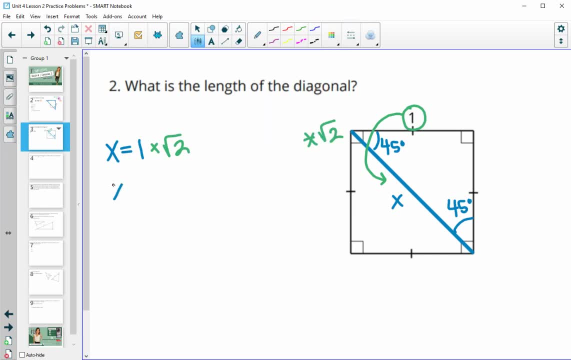 So x is just going to equal square root of 2.. You can also, if you like better, you can- use that parent triangle idea. So let me just draw this parent triangle over here also and give you one other strategy. So if we have this parent triangle and you can remember on a 45-45-90 that that means that the legs are 1s and the hypotenuse is a square root of 2,. 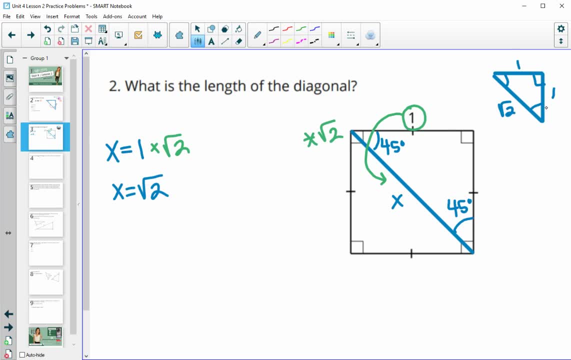 then you can also set up proportions. I mean, and if you recognized this, this one just has 1 and 1 over here, And so then that would have to be square root of 2. But you can also set up proportions. 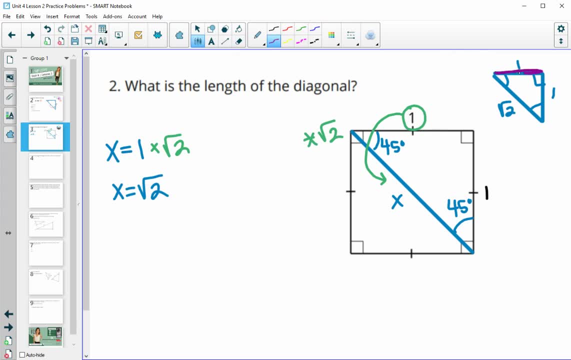 You can also match the corresponding side. So this one's a 1.. So I would put a 1 underneath this one And then the hypotenuse is a square root 2.. So I would put a square root 2 under this x and then set those equal to each other. 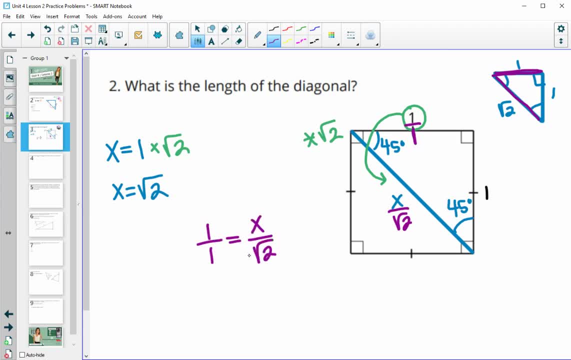 So 1 over 1 equals x over square root 2. And then you'd be able to cross multiply And you'd get square root of 2 equals x that way. So you can also set up proportions with similar figures, if you'd rather. 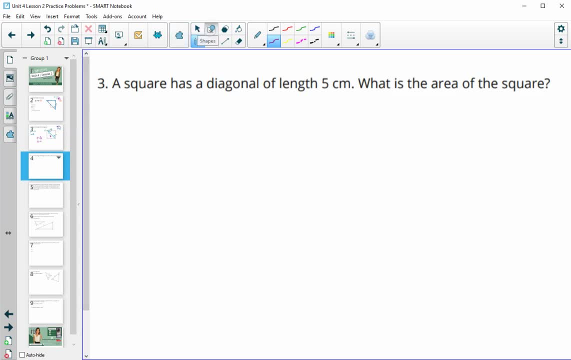 Number 3, a square has a diagonal with a length of 5 centimeters. What is the area of the square? So we know this diagonal here is 5.. We also know that the legs are all the same in a square, So we have two 45-45-90 triangles. 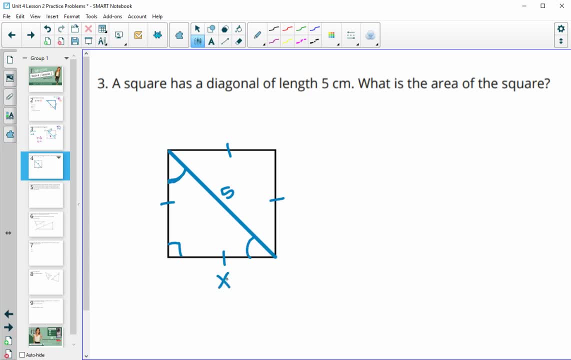 And so we just need to find one of these legs, And then we're going to do that, And then we'll know both in order to do the area. So area formula for a square is just to take one of the sides and square it. 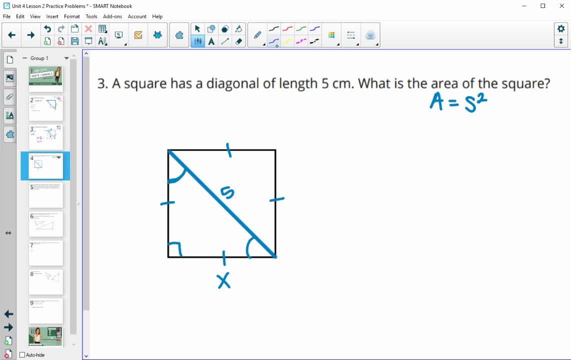 because it's just base times, height and the sides are going to be the same. So let's take a look again if you want to be looking at that parent triangle To help you. we've got each of these side lengths being a 1. 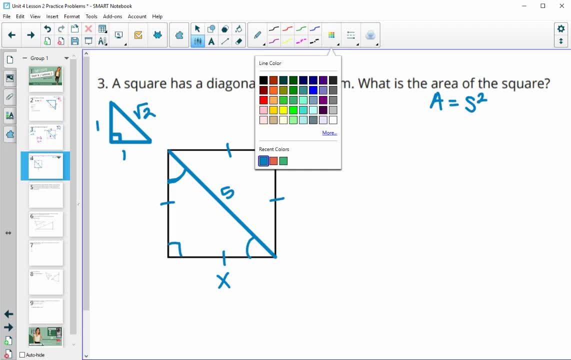 and then the hypotenuse being a square root of 2.. So remember, in this, when we have the hypotenuse and so to get to the leg, we would just divide by square root 2, if you want to be doing that. 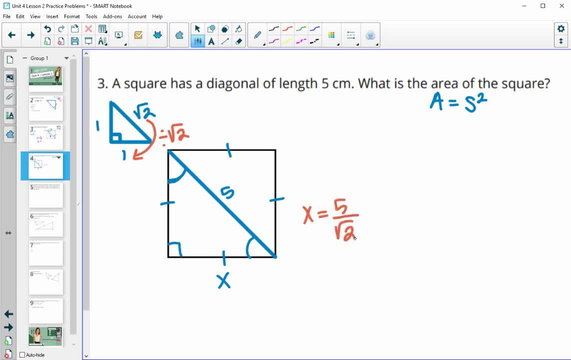 So x is just going to equal 5 divided by the square root of 2.. And so that's what each of these sides are. And so then we're going to do the area formula, And the area formula is going to take the side 5, square root of 2,. 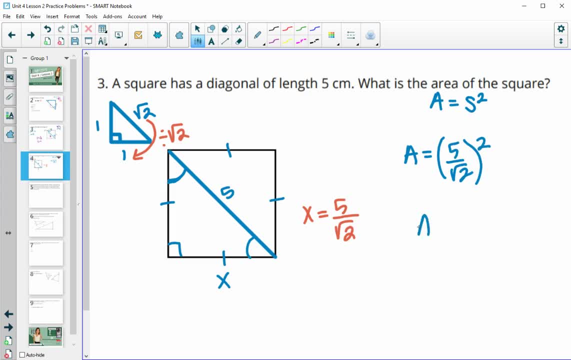 and it's going to square it or multiply it by itself. So in this case, 5 squared on top is 25.. And then the square root of 2 squared is just a plain 2.. So it looks like this: Square root of 2 squared. those will just cancel and you'll get a 2.. 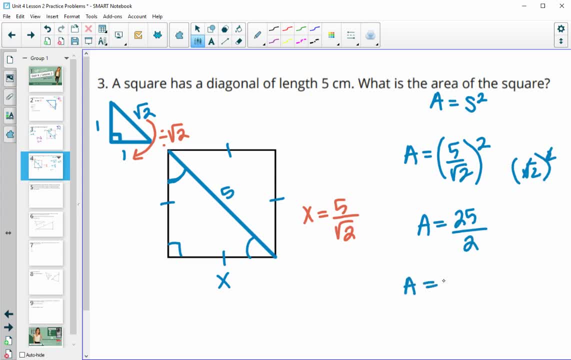 And so you can leave it like that, Or you could do 25 divided by 2 and get 12.5 units squared, or centimeters squared in this case, because they actually told us that it was 5 centimeters. And then, if you want to do, 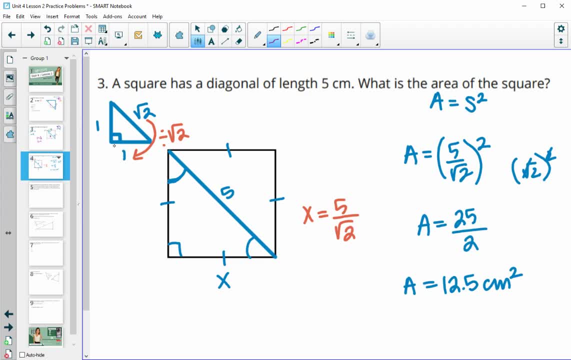 that proportion method. this is maybe a better one to show you. So this leg is 1.. So on the leg, I'm going to put that over 1.. And then the hypotenuse is a square root 2.. So I'm going to match that square root 2 with the 5.. 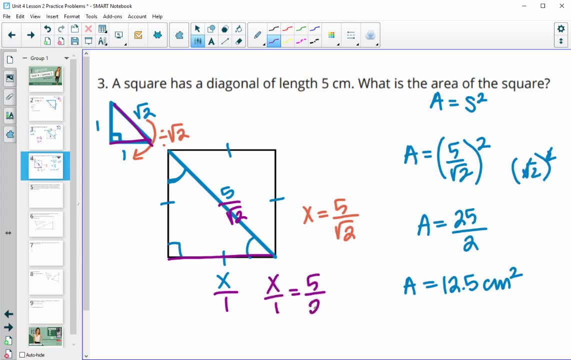 So then you would have gotten: x over 1 equals 5 over square root 2. And we know, anything divided by itself doesn't change it. So then you would have ended up with 5 over square root 2 for the side length. 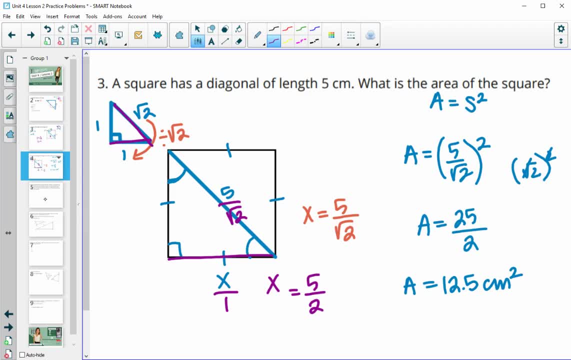 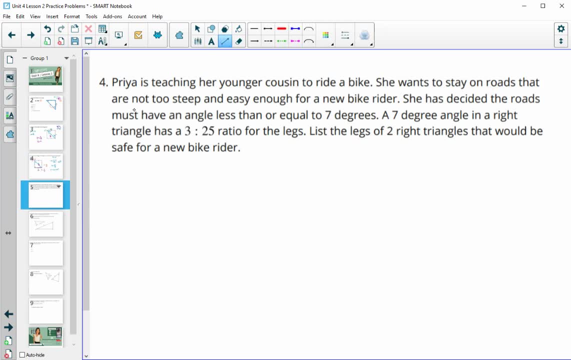 just like we did this way, squared it for the area Number 4,. Priya is teaching her younger cousin to ride a bike. She wants to stay on roads that are not too steep and that they're easy enough for a new biker to ride. 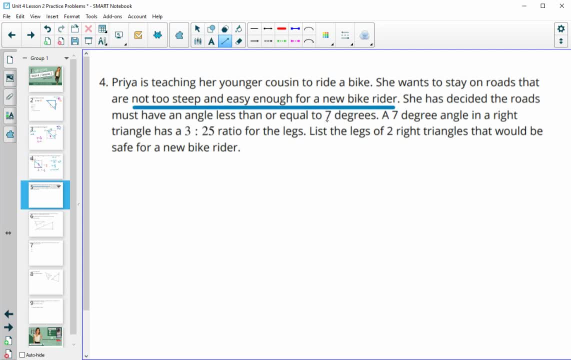 So she's decided that roads must have an angle less than or equal to 7 degrees. And she knows that a 7 degree angle in a right triangle has a 3 to 25 ratio for its legs. So list the legs of two right triangles that would be safe for a new biker to ride. 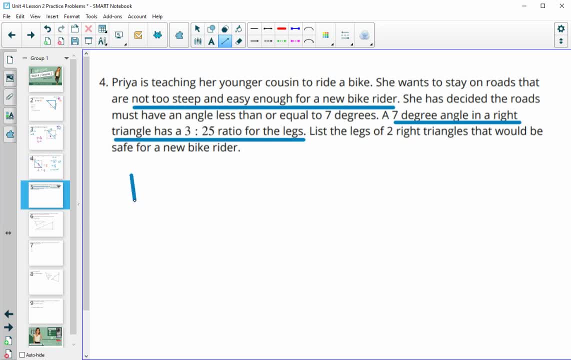 So I'm just going to draw out a 3 by 25.. So if the height is 3,, then the leg would be 25.. So it would be something like this: And now, in order to keep this angle smaller, either you could just leave the 25 the same. 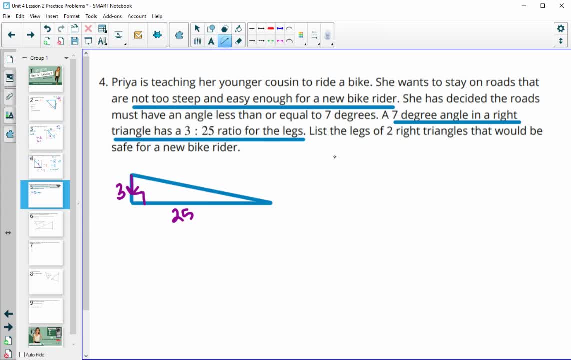 and then the height just needs to get shorter so that that angle decreases. So you could do something like 2 by 25.. So that's certainly going to get a smaller angle, So a 2 by 25.. Or we could leave the height the same and just extend this length. 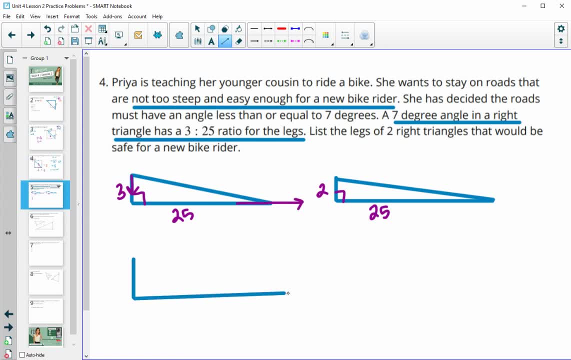 So if we left the height at 3, then we would just need to extend this further. That's going to pull that angle to be a smaller angle as well. So you could leave this at 3, and then you could put this leg at something like 26 or higher. 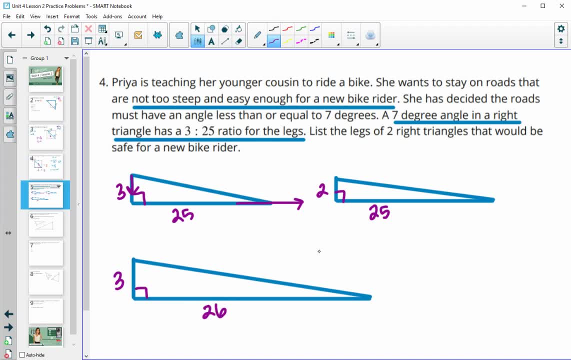 So that will kind of guarantee it. If you wanted to change these measures and then check, just make sure you look at 3 divided by 25.. So that decimal which is 0.12.. And then you compared your height divided by your length. 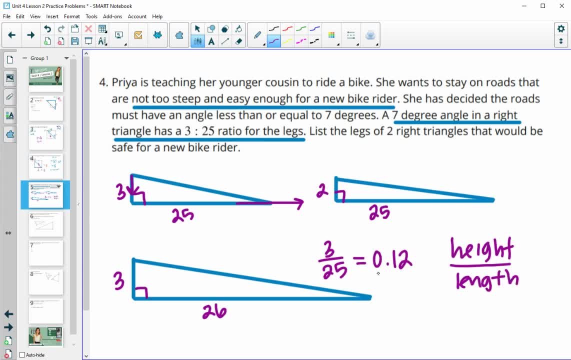 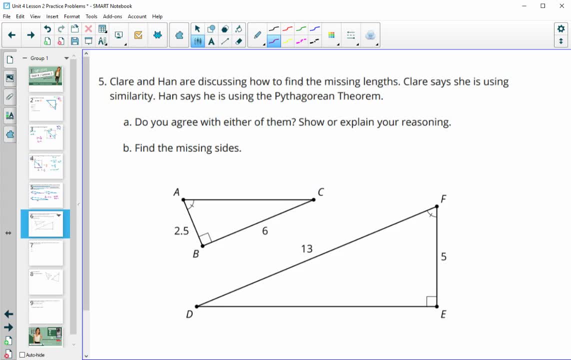 And you just make sure that that's less than or equal to that 0.12.. Number five: Claire and Han are discussing how to find missing lengths. Claire says she's going to use similarity and Han says he's using Pythagorean theorem. Do you agree with? 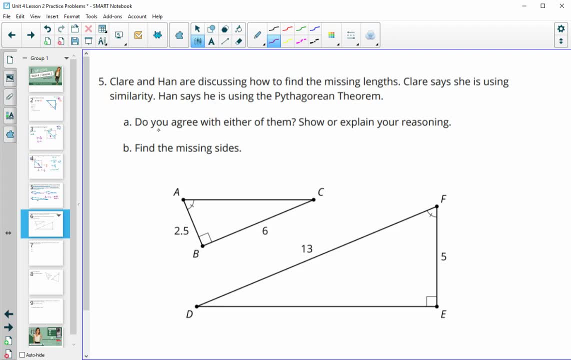 either of them and show your reasoning, And so they're going to find the missing lengths of both of these. So for Pythagorean theorem we have to have a right triangle, and we do have a right triangle in both cases, with two of the legs given to us. So here's the right angle, and then 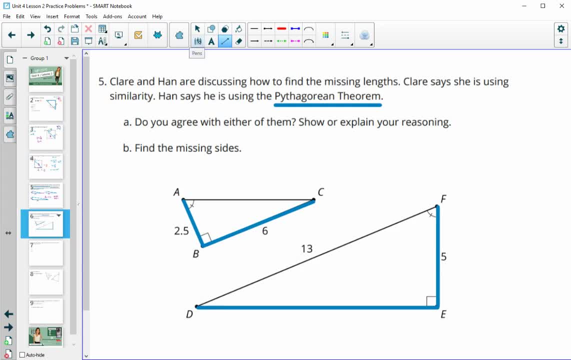 two of the legs are given here, So Pythagorean theorem is certainly going to work. So I will do that. on triangle DEF: So we're given the hypotenuse is 13.. So 13 squared equals 5 squared plus ED. squared So, 169 equals 25 plus ED. 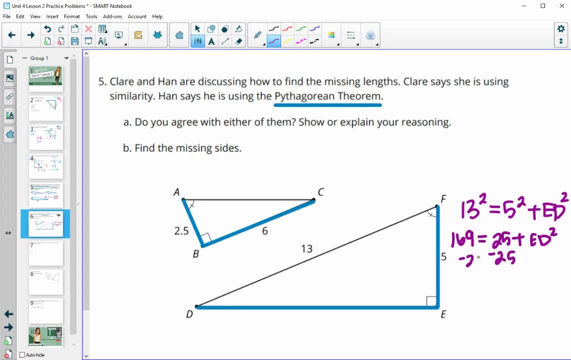 Subtract 25 and we get 144 is equal to ED squared, And then we'll square root and we get 12 for ED. So that is a totally fine way of doing it, And you can certainly do that with this one as well. Do 2.5 squared plus 6 squared equals AC squared, And then we can in fact also: 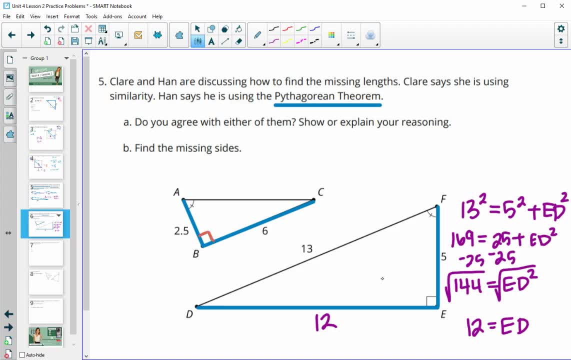 do similarity Because they share two angles. So we've got a right angle that's equal to each other and we've got this angle marked as congruent, So we know that the two triangles are similar, So we're going to be able to use similarity as well. So this height kind of here, this short leg, 2.5 goes. 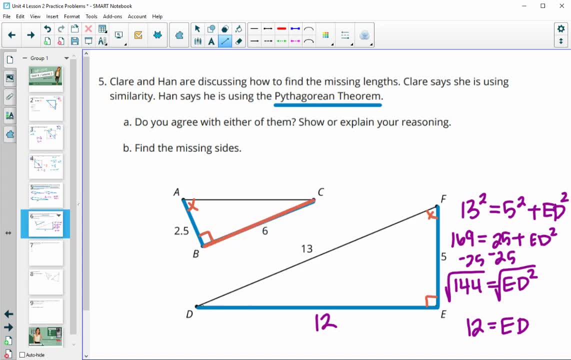 with the 5. And then this longer leg 6 goes with this longer leg of 12. And so that shows us that we actually have a scale. So now, if I'm going to go 13 back to this way, I want to look at taking the 12.. How do we go? 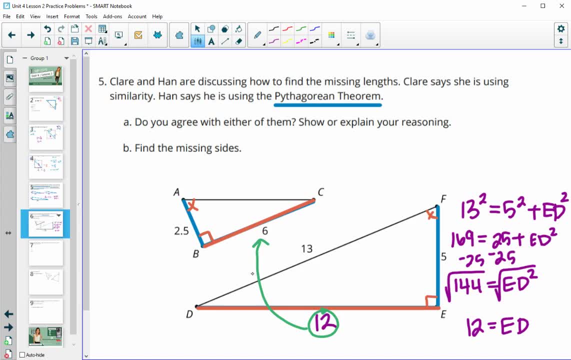 from 12 back to 6?? And so you can think of that as multiplying by 1 half or dividing by 2.. So I can take this 13,, divide it by 2, and that will give me this side of 6.5.. So either way that you do this, 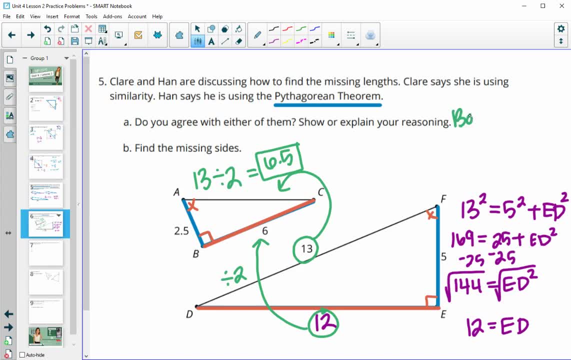 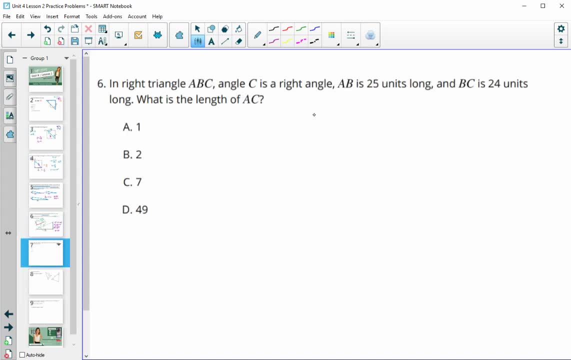 you could do similarity Or Pythagorean theorem, So I agree with both of them. Number 6: in a right triangle, ABC, Angle C is the right angle. so let's draw out a picture of a right triangle here. So angle C is the right angle, And then you can label A and B, whichever other ones you 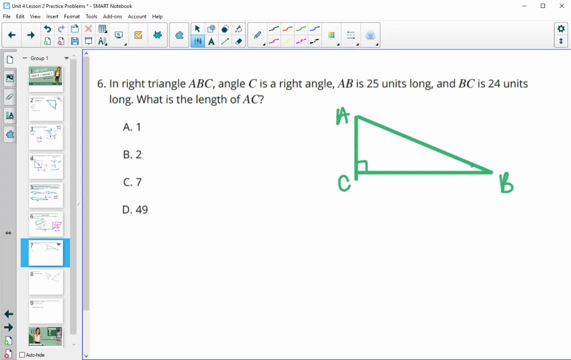 want, And it says that AB is 25 units, which is our base value, And it says C is 25 units. That's what you're doing, So so much waiting. Now we need to figure out how many angles are we going to make of these angles? So, based on the 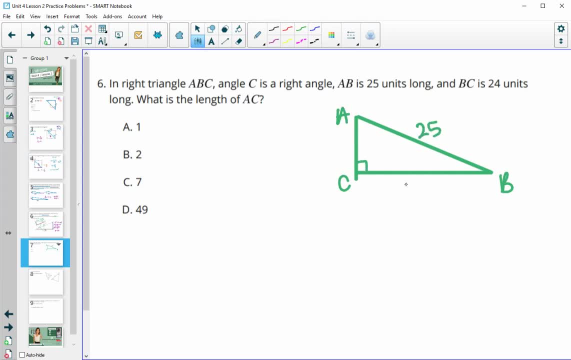 additional details of the two triangles here. I'm going to just go ahead and just take each angle and add them and multiply them 10, and then I'll just do another one 10, and then I'll just do another one. long, and BC is 24 units long. what is the length of AC? So, since it's a right triangle with two, 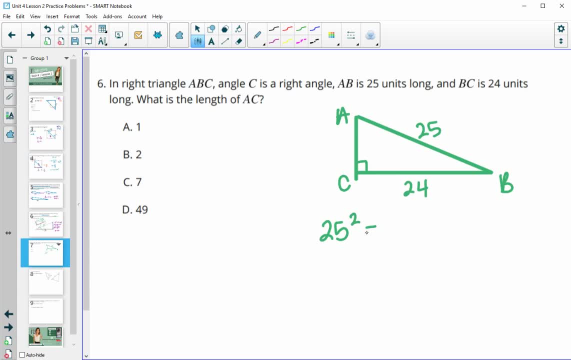 legs given. we know we can do Pythagorean theorem. So we square the hypotenuse and then we square both of the legs and add them together. 25 squared is 625.. 24 squared is 576.. And then we have that. 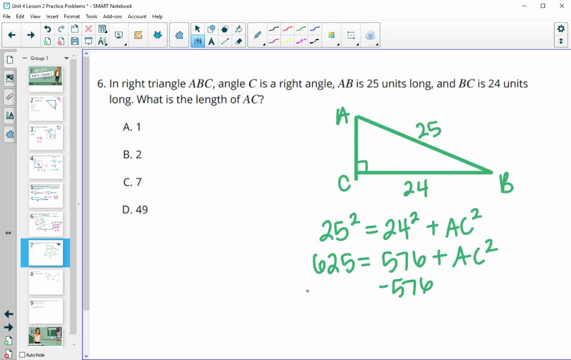 AC squared. Subtract the 576 from both sides and you get 60.. No, what did we get? 49. Okay, so 49. And then we have that AC squared, And then we will square root both sides and get 7 for the length of that missing side. 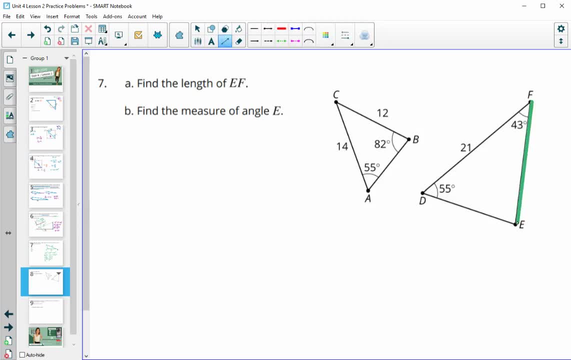 Number seven find the length of the hypotenuse. So we're looking for this side length, And so we got to make sure that these two triangles are similar before we do anything, since we only see this 55 degree angle in common. So let's first. 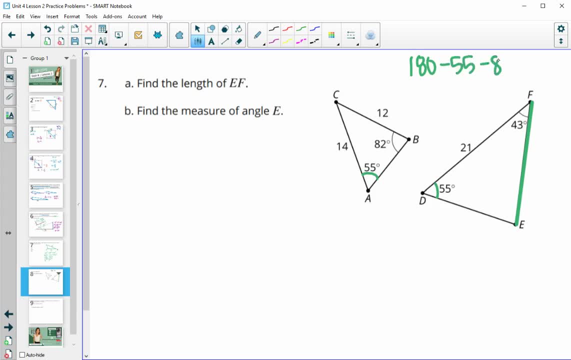 do 180 minus 55, minus 82 and find out that we get 43. So this angle here is equal to 43, which we also see here. So we know for sure that we can do similarity. And then let's kind of match up some of these. 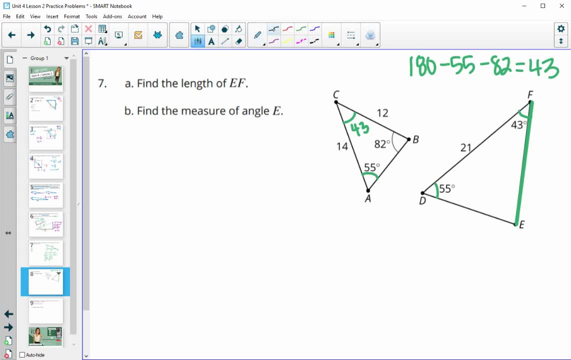 sides. so EF is the side that connects 43 to the 82 degree angle, And so we can mark that here the 43 to 82 is BC. Then we also see this 21,, which connects the 43 and the 55. And over here we see the 14 is the 42 degree angle here. 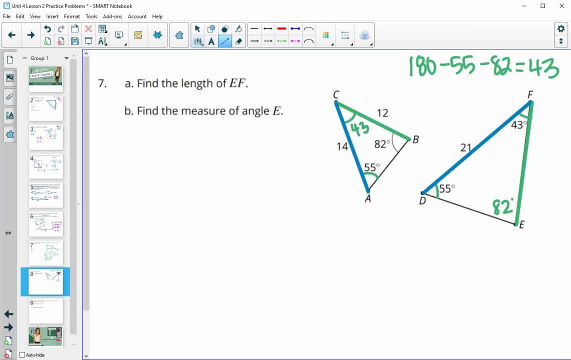 is the side that connects the 43 and the 25, and so those sides are what we're gonna use to set up a proportion, or you can do scale factor if you would like. so I'm just going to do proportions in this one, so EF. so I'm going to compare side. 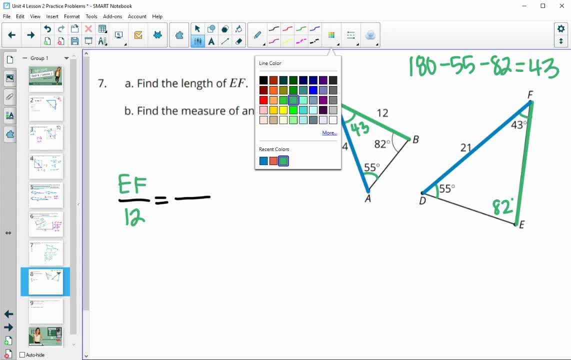 EF to 12, and then we can compare 21 to 14, and then we'll be able to cross multiply here, and so we'll do 12 times 21, which is 252, and then we will divide that by 14 and we will get 18. so EF equals. 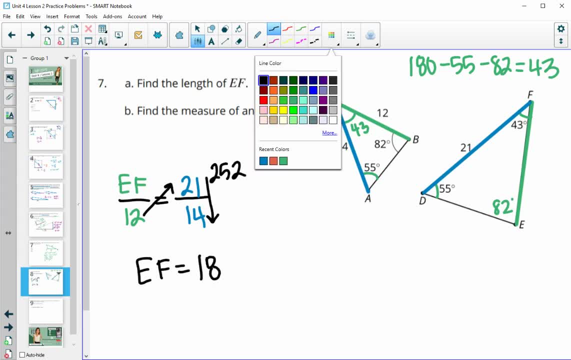 18.. And again, you could have used scale factor here as well, so you could have looked at what do we do to the 14 to get to 21. so that's 21 divided by 14, which, if you wanted to simplify those, both divide by seven, and so that would. 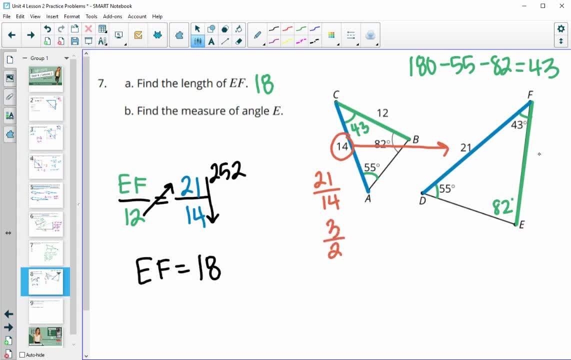 simplify down to 3 over 2, so then this EF is going to be 12 times 12, and then EF equals 18.. So this would have been a little bit more simple. So that would have been the same thing, but it would have been a little bit more. 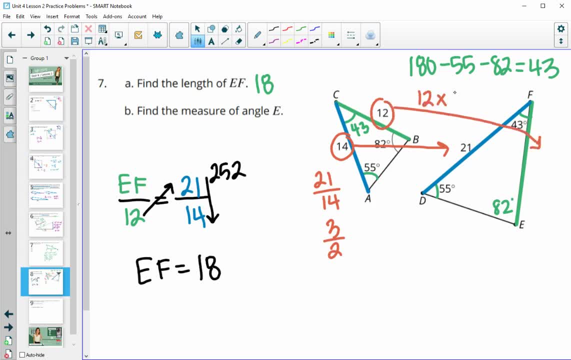 the scale factor. So we're going to do 12 times three halves or times 1.5, and that's going to give us 18 that way as well. And then angle E- I actually already wrote in- and that is 82 degrees. 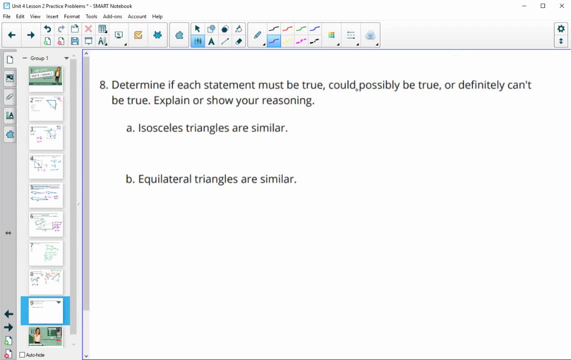 Number eight determine if each statement must be true or could possibly be true. Isosceles triangles are similar, So we certainly can get some isosceles triangles that are similar. So if I did this- here's an isosceles triangle- I could mark these sides the same, And if I just grouped 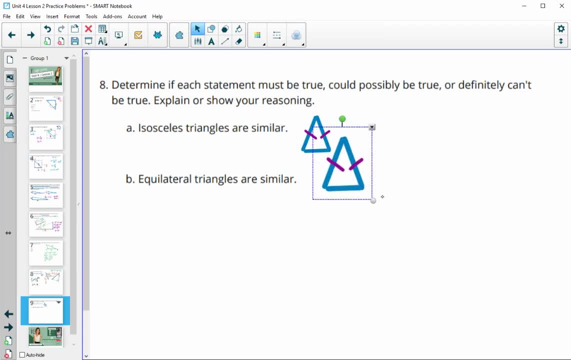 these on my page and then I duplicated it and made it bigger. these are going to be similar to each other. I just dilated it. So certainly we can have isosceles triangles that are similar, but all isosceles triangles don't have to be, because I could draw this one. 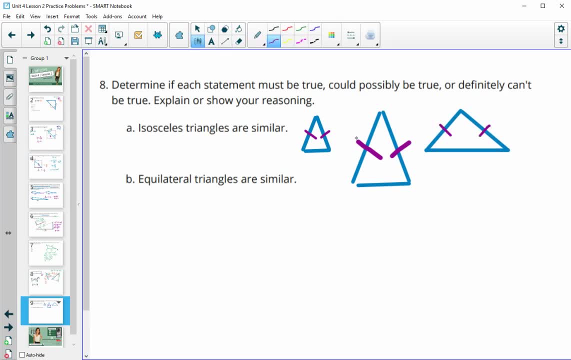 and this one is certainly not similar to these ones, because this is an obtuse or a much bigger angle than this one. So this could be true, but does not have to be true For equilateral triangles. okay, equilateral triangles always have to be similar, And that's because all three sides are.